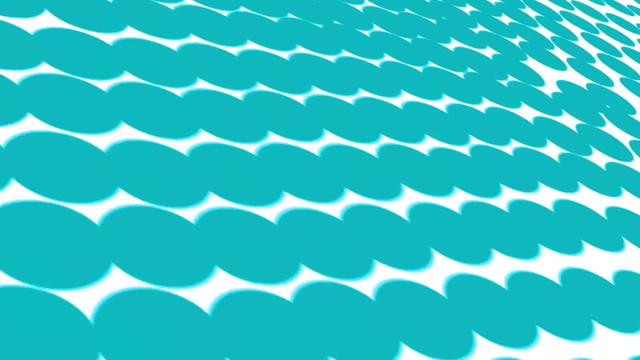 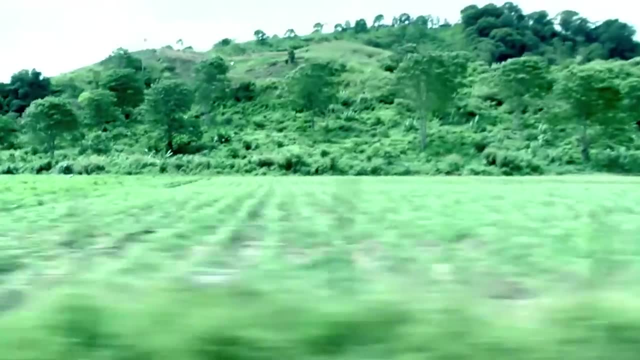 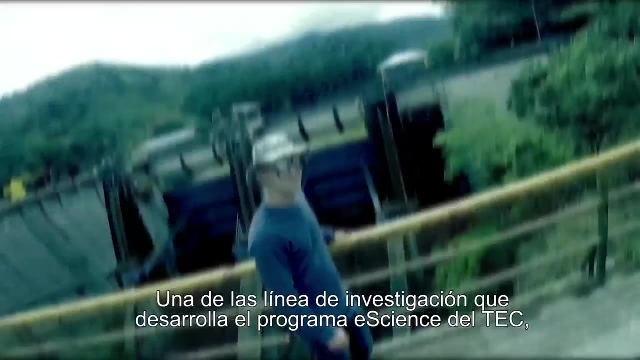 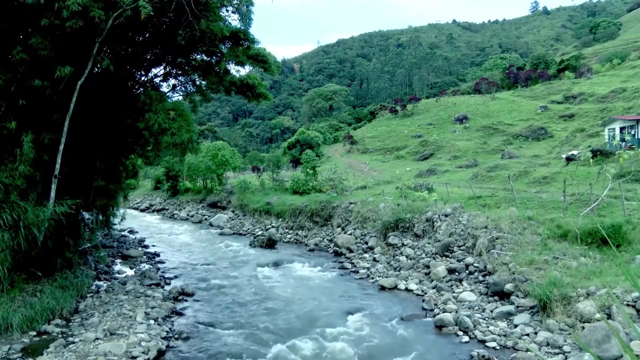 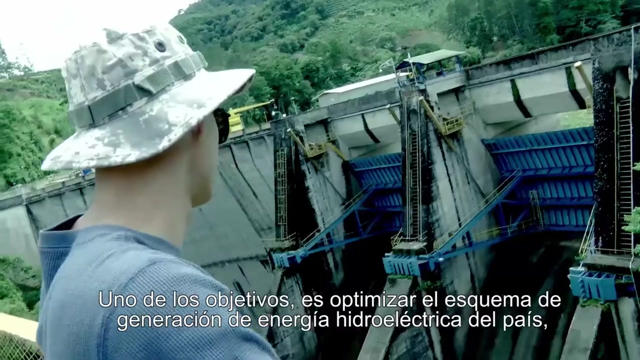 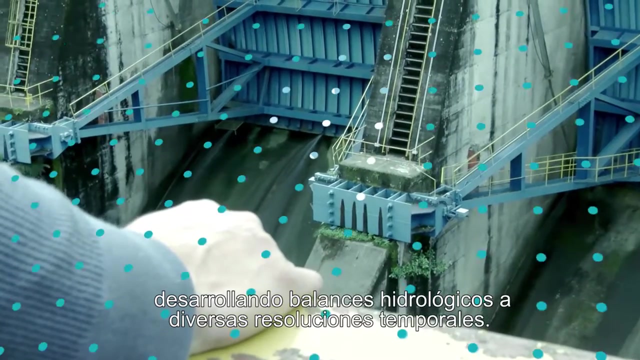 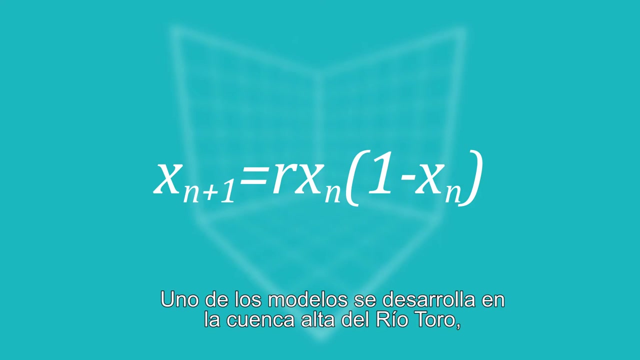 One line of research developed at TECH's e-Science program is Hydrological Modeling and Climate Change. One of the research objectives is to optimize the national hydropower generation framework by developing water balances at various temporal resolutions. One of the models, the HBV-TECH, is being applied to the upper Toto River catchment. 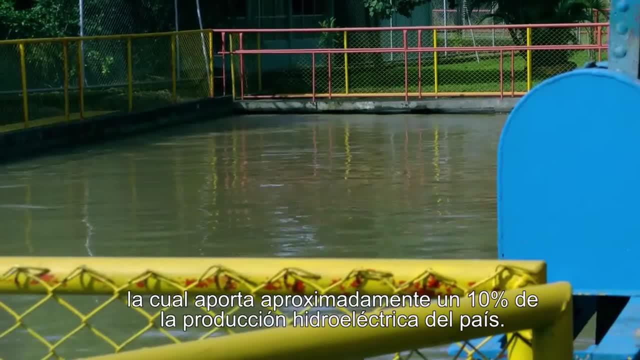 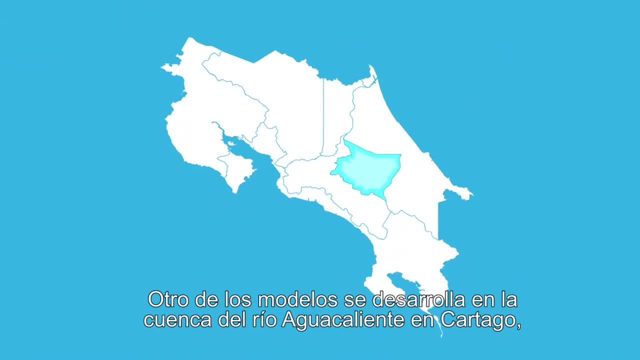 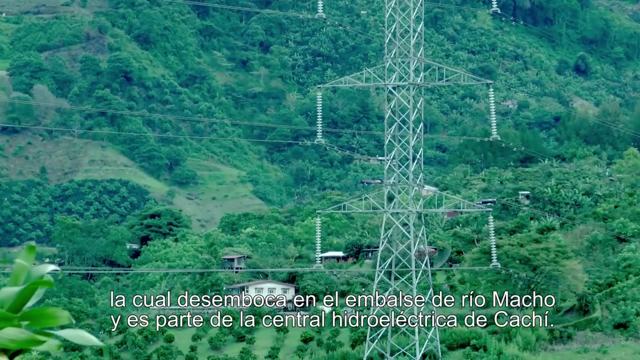 which contributes with approximately 10% of the national generation. The model is also being applied to the Agua Caliente River catchment located in Cartago, Central, Costa Rica. At the same time, this catchment flows into the Rio Mach Reservoir, which is part of the 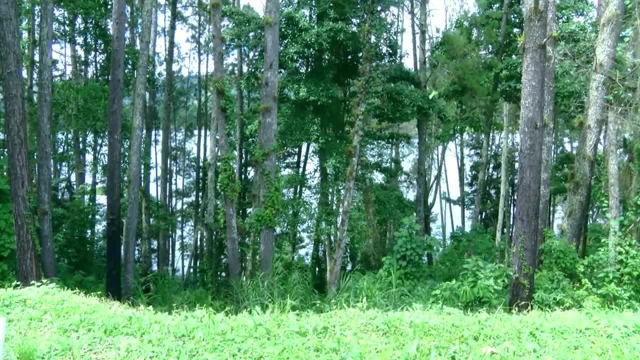 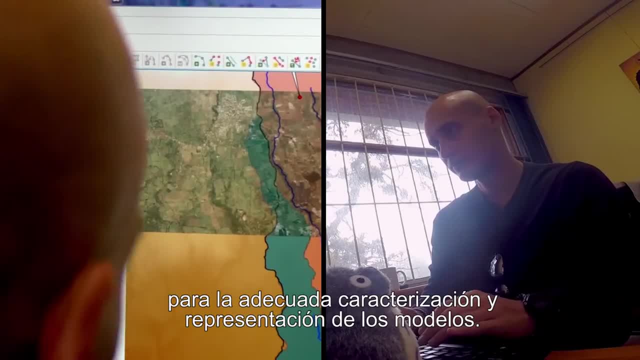 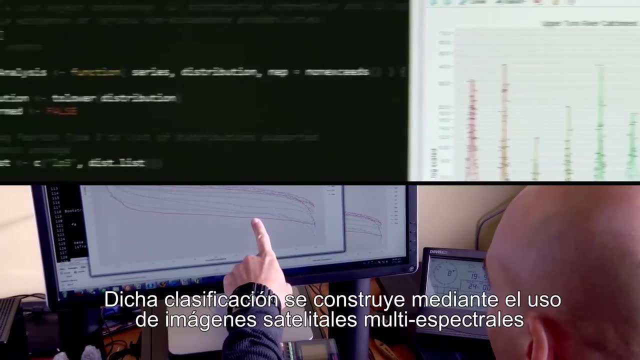 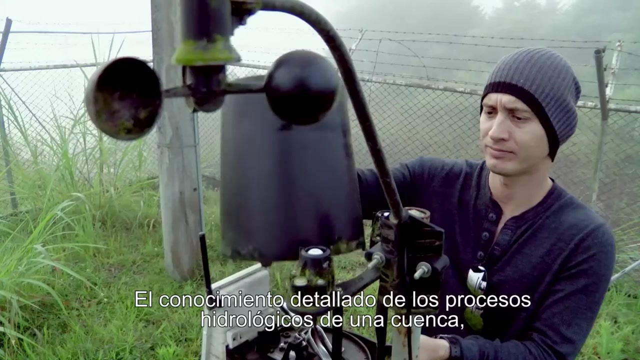 Cachí hydropower plant. In both cases, the detailed classification of land use is essential for an appropriate characterization and representation. Land use classification is developed through multispectral high-resolution satellite imagery and field validation. A profounder knowledge of the hydrological processes of a basin is essential for both. 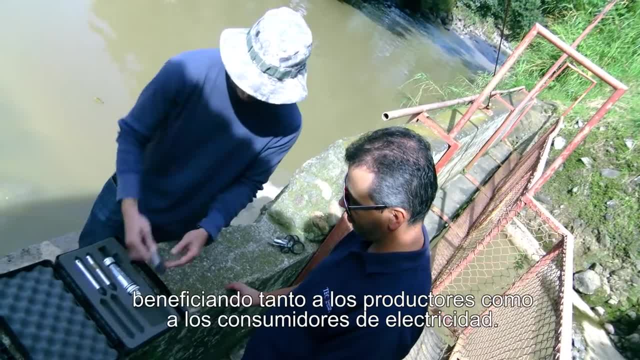 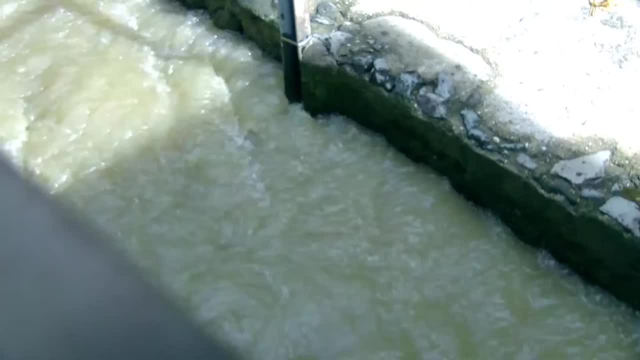 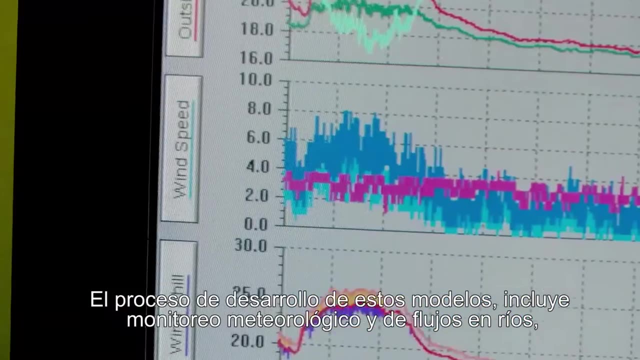 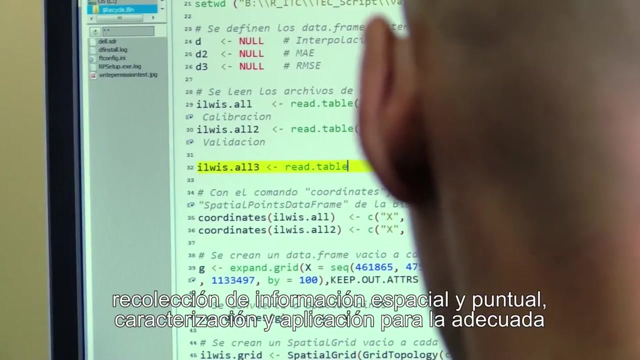 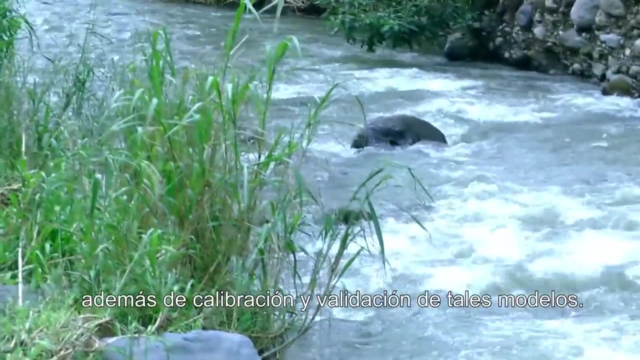 producers and consumers of electricity and in the operation and projection of the hydro-electrical potential of the catchments. The development process of the HBV-TECH is based on the development process of the HBV-TECH and the HBV-TECH's. 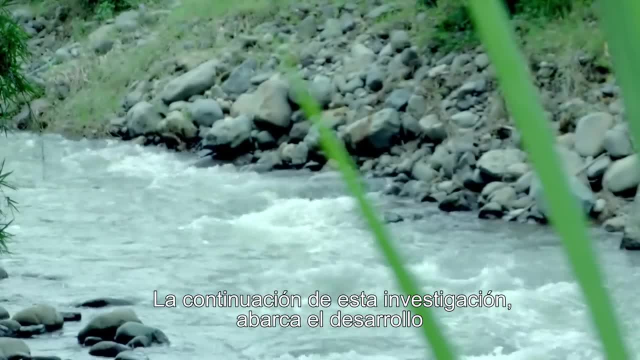 HBV-TECH. The development processes of these models includes meteorological and river flow monitoring, gathering of spatial and punctual information, characterization and application for an accurate representation of the different physical processes of the basin, in addition to calibration and validation of such models. 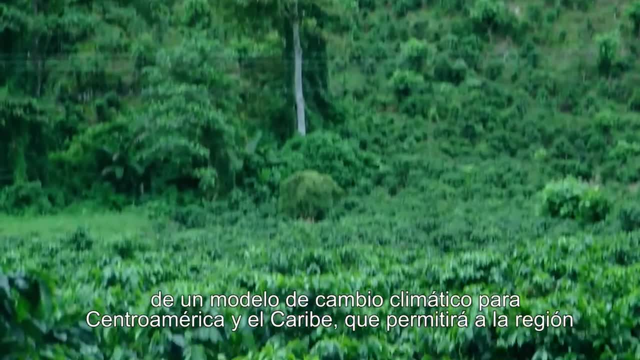 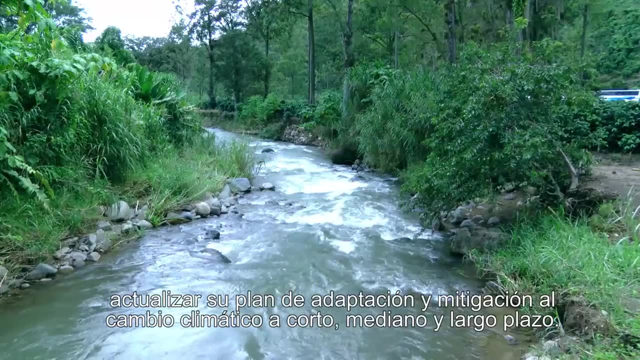 The continuation of this research comprises the development of a climate and water environment and the development of the HBV-TECH. The HBV-TECH is a climate change model for Central America region and the Caribbean, which will allow the region to update its adaptation and mitigation plan in the short.